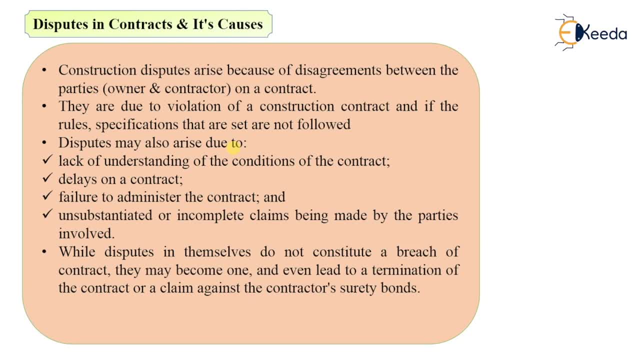 the special slides. but let me tell you what are the basic causes of disputes, see lack of understanding of the conditions of the contract. there are chances that some of the conditions are there in the contract but maybe owner has not understood that condition, maybe contractor has not understood that condition. then if there are delays on a 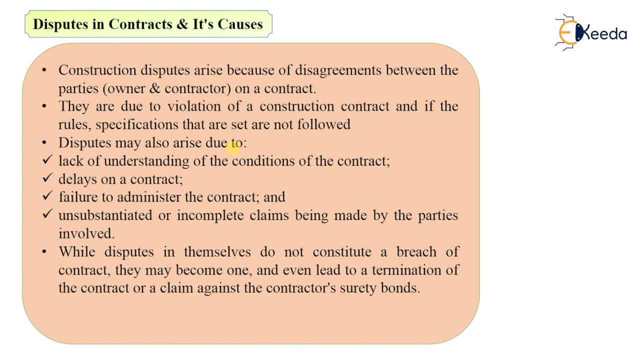 contract. if the contract is not getting completed within the prescribed time, within the prescribed schedule, then in that case there are chances of arising of disputes. then failure to administer the contract: if the contract is not administered properly, if it is failed to administrate the contract, then in that case dispute may arise. 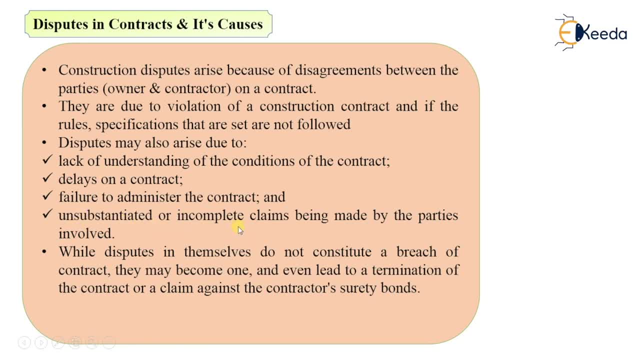 then unsustain sustantiated or incomplete claims being made by the parties involved. see, there are certain claims that are made, if they are made by the parties, may be by the owner, may be by the contractor, and in that case there are chances of disputes. for example, there was not mentioned that 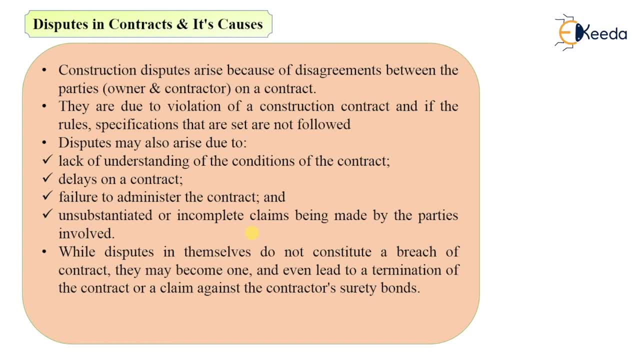 construction of this. this particular part was there or not, but owner says that it was included in that. so there are chances of disputes then. while disputes in themselves do not constitute a breach of contract, they may become one and even lead to the termination of contract or claim against. 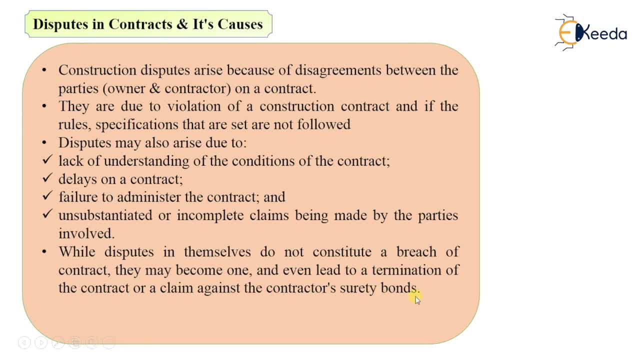 the contractors surety bond. see this point. I will explain you in detail what it says. disputes will not reach the contract. it will not break the contract, but it may become the reason to break or bridge the contract. are you getting or not? it is not the that if there is dispute happening, 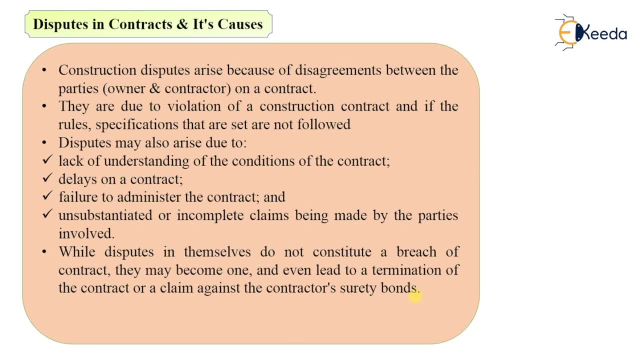 if any dispute is happening between the contractor and the owner, between the parties, then contract contract will be breached. it is not like that. it may still continue, but it may be the biggest reason. if dispute is happening between owner and the contractor, why should contract be continued? so it will get terminated. the contract gets terminated, it will lead to the termination of. 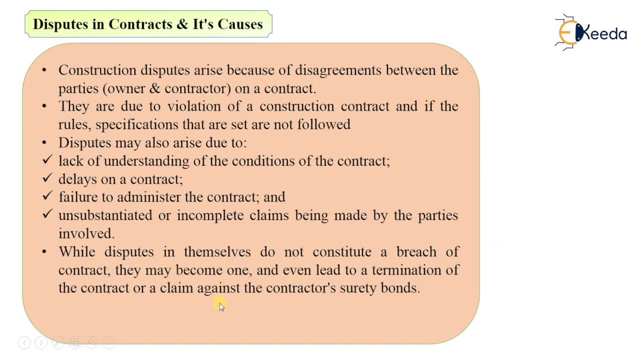 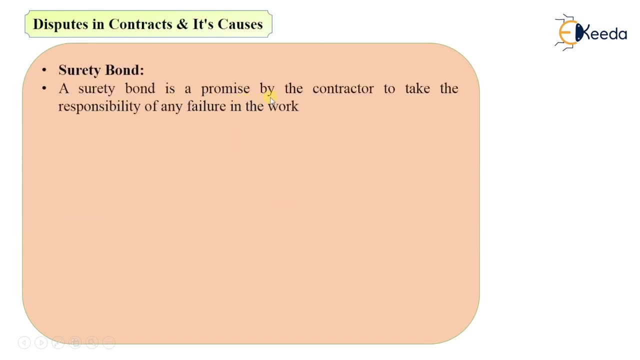 contract if any dispute happens between the owner and the contractor. and there is one concept here. she see, i have told you claim against the contractor's surety bond. now what is surety bond? let me tell you first what is surety bond. see, a surety bond is a promise by the contractor to 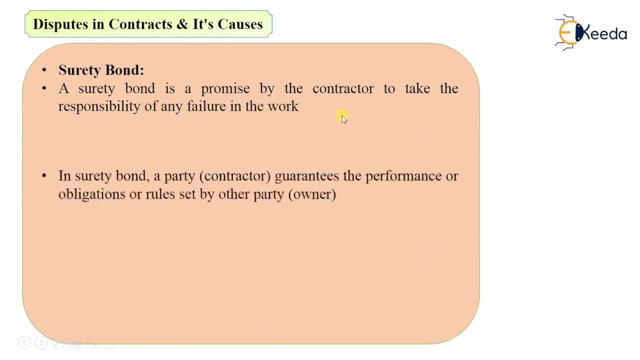 take the responsibility of any failure in the work. in return form he will sure give surety to the owner that if any failure happens in the work, if i am not, if i am not able to complete your work within the prescribed time, if the work is not done as per the specifications, then i will be the responsible person that that. 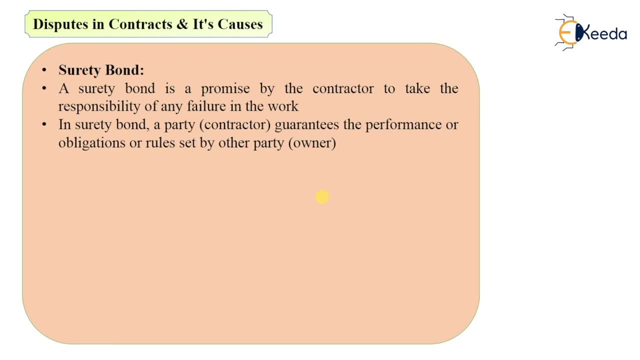 is what written in the surety bond by the contractor and he will give it to the owner. so in surety bond a party party is who. a contractor guarantees the performance or obligations or rules said by the other party, that is, owner. owner will set some of the rules. 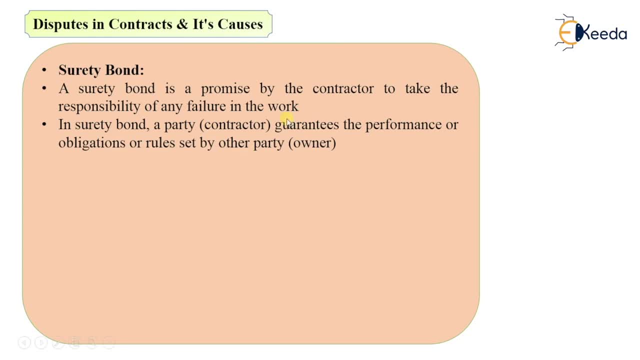 regulations, specifications of the work and contractor will guarantee that i will follow these rules and regulations and obligations which you have set. so that is the surety bond. okay, and surety bond is a third party contract comprised of surety, the principal, and the oblique- oblique- see, oblique means the owner, principal means the contractor. so the contractor. 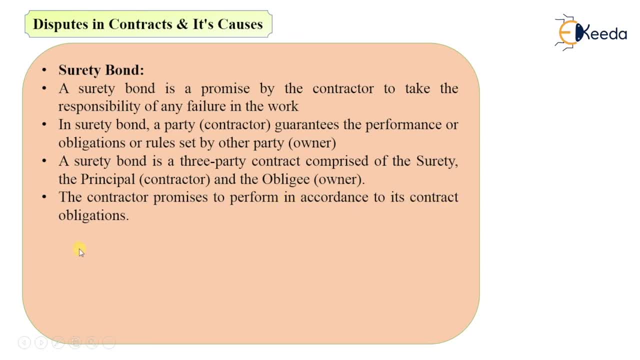 promises to perform in accordance to its contract obligations. it is simply the promise made by the contractor to take the responsibility of any failure in the work. he will guarantee the performance of work. he will guarantee that i will follow all the rules and regulations which you have said. so that is called as your surety bond and 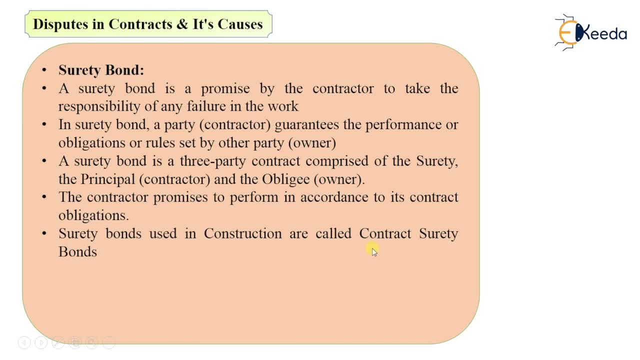 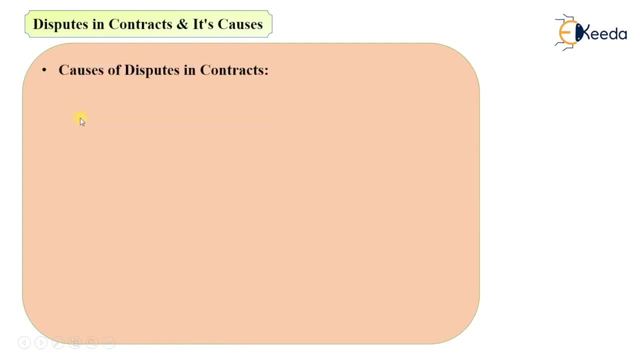 it is also called as in the construction field. it is also called as contract surety bond. remember this. so we you got the idea. now let's see what are the causes of disputes in the contract, why dispute arises between the owner and the contractor. see, the first cause is contract errors or omissions of items of work means if there is omission of 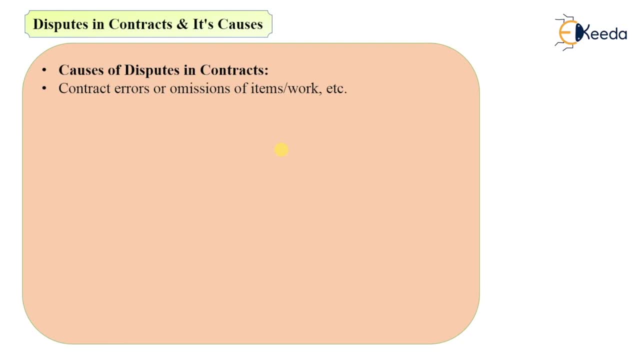 the a particular quantity, a particular work, when contractor has not completed, he has omitted some of the quantities, some of the items of work and he has not completed that, he made some errors in that particular item of work, then in that case dispute may occur or arise. then deferring site. 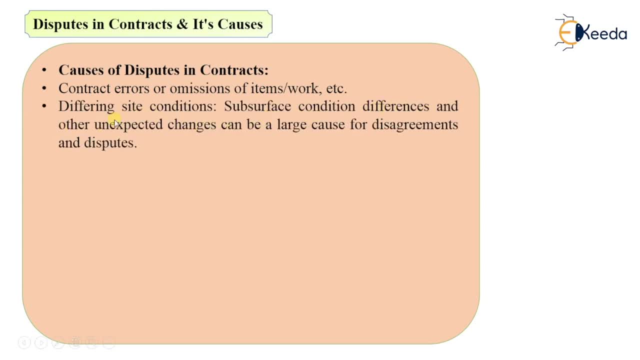 conditions, subsurface condition differences and other unexpected changes can lead or can be a large cause for the disagreements and disputes. for example, the contractor agreed to work for a certain amount for the excavation by the safe for by the excavator by manual excavator. maybe he will. 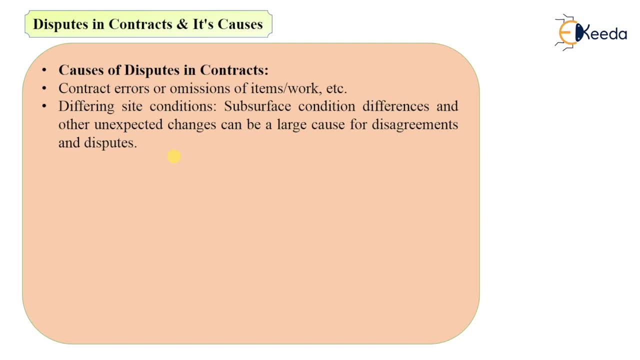 be using manual excavators or he will be using jcb. so he agreed to that. but subsurface conditions: he found that site conditions are not like that which he was expecting. the site is too hard, the stones are too hard, the jcp will take so many hours to uh dig that particular pit or trench. so in that case he 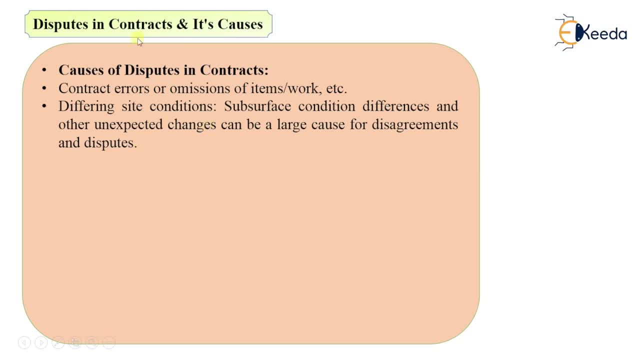 will not accept the agreements and there will be dispute between the owner and the contractor. then non-compliance of the contractual obligations: if contractor, even the subcontractor, or employer or any other party, fails to comply with their obligations, the other parties which are involved will generally try to seek the recourse. what he will do for. 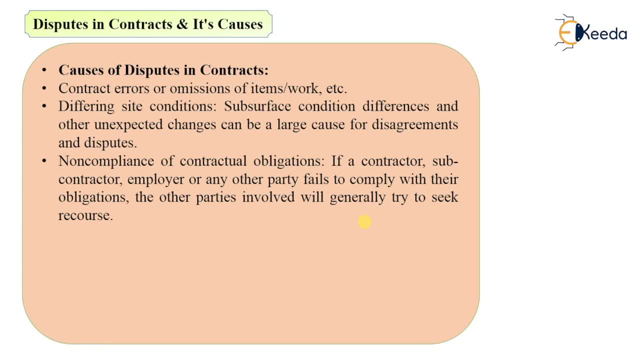 example a contractor, say contractor is a one party. so if contractor is not following all the rules and regulations which are there in the contract he is not following, he is not complying with the rules obligations made by other party, that is, the owner. so there will be chances of 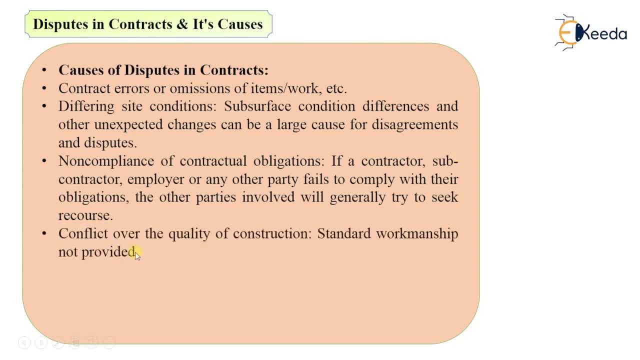 arising. the disputes then conflict over the quality of construction. this is one of the most most important causes of disputes: that quality construction is not achieved or it is not given by the contractor. standard workmanship is not provided, he is not using proper workmanship, the work is not up to the mark. very poor workmanship is there then in that case? 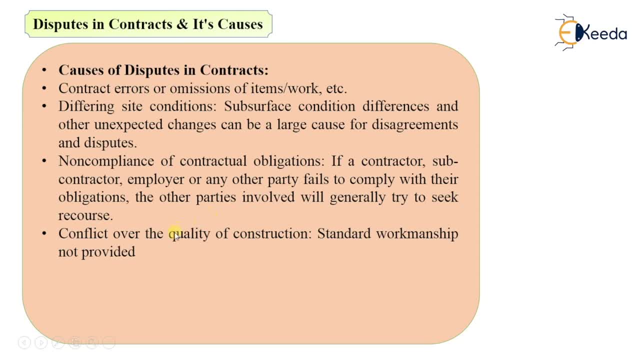 obviously owner will get the quality of construction which is not given by the contractor angry and there will be dispute, then conflict over the material, see, there will be workmanship errors and there will also be conflict over the materials if contractor fails to use the materials that are specified in a contract. if he fails to do so, for example, first quality brick first. 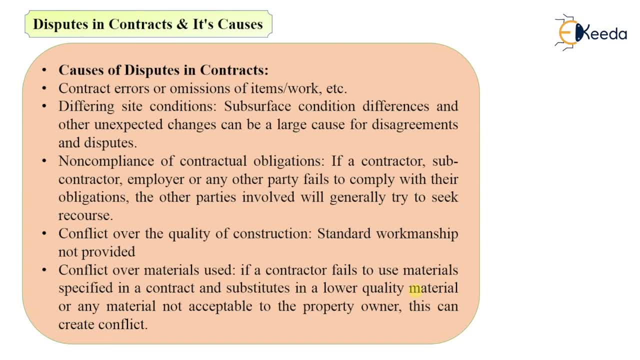 class brick work was mentioned, but he is using another brick that is not up to the mark. that is not a very good quality brick. then there will be dispute. if he mentioned that this, this pint, i will be applying plastic paint, i will be applying in the hall, but he's not applying the plastic paint. so, materials over the materials, there will be a. 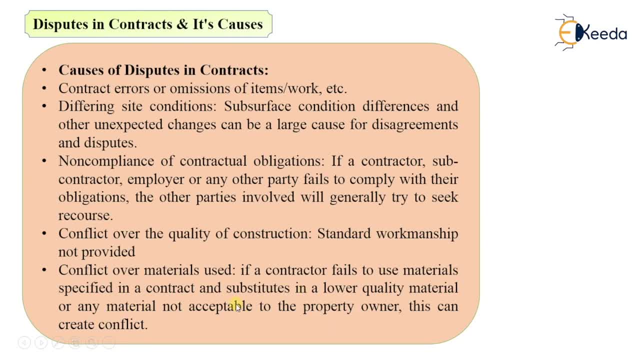 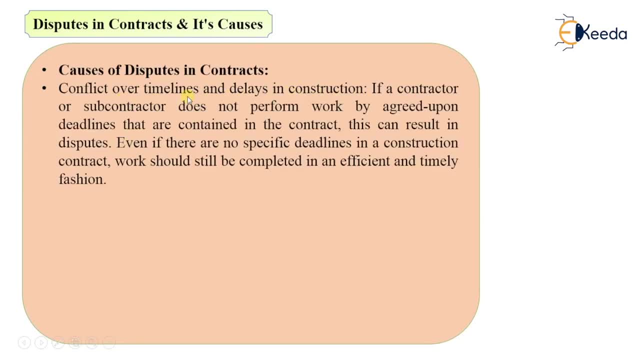 big issue and dispute between the owner and the contractor then conflict over timelines and delays in the construction. this is also one of the important or biggest problems or causes of disputes if contractor or subcontractor is not completing the agreed work. in theford, we ask for pre- bracelets and winooooooooooooooooooooooooooooooooooooooooo. 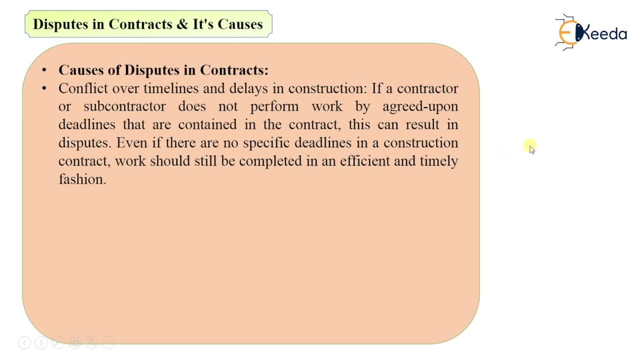 buy in the cart. so we ask for pre-brackets. then the cost is very heavy because price is very much higher than expect. these are impatient car dealers, even if this is very expensive. repaired line minimalist. sir, why aren't you doing so? make them copy the black art houses. 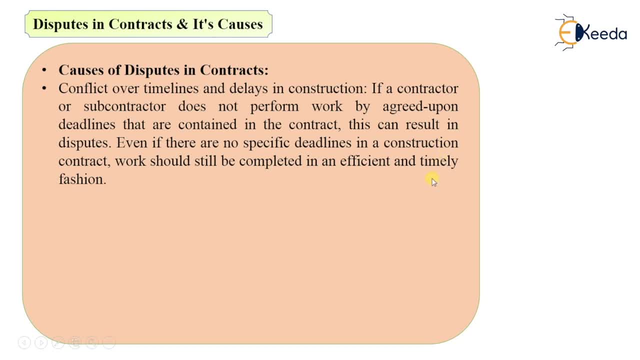 Нет ca da da that he knees overivoics tha we do. american contrast art fabric. did i get hat done in the past? deadlines within prescribed time limit, within the schedule, then there are chances of causes of, then there are chances of arising the disputes. for example, deadline is any date, any date. 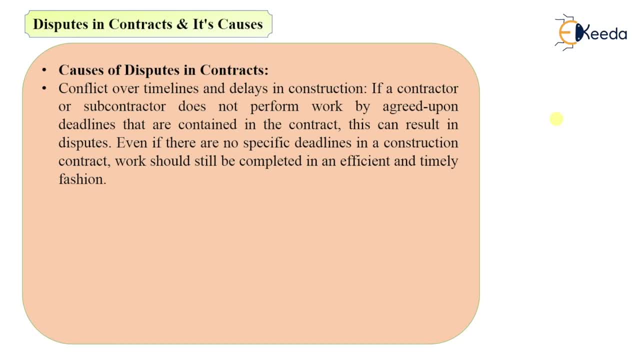 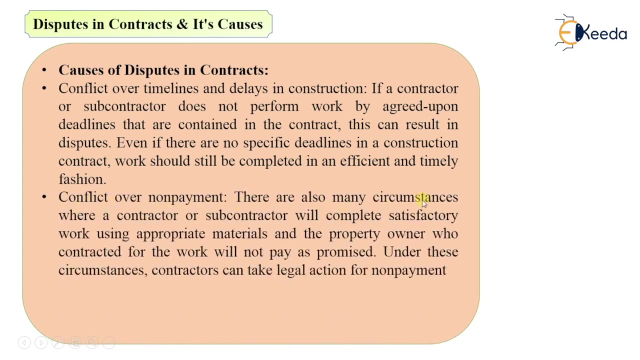 and he is exceed exceeding that work maybe by 15 days, then it is okay, but he is not completing the work for many months, even after the deadline, then there will be chances of disputes, then conflict over non-payment. there are also many circumstances, see when contractor or subcontractor will complete. 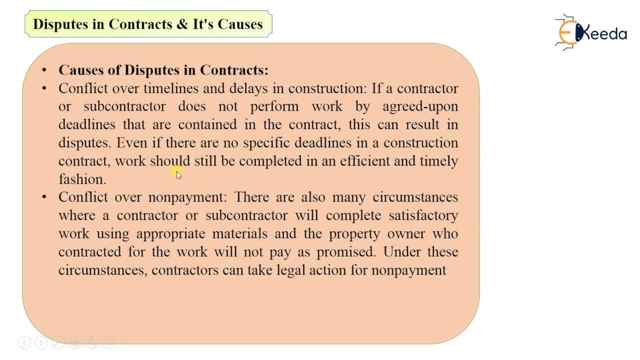 the satisfactory work. it is not like always. the problem will be from the contractor. some of the times, what happens? even the contractor or subcontractor will do the work very properly, very satisfactorily. but what happens? owner will not pay him as promised. so under these circumstances, contractor can take the legal actions for the non-payment and there will be. 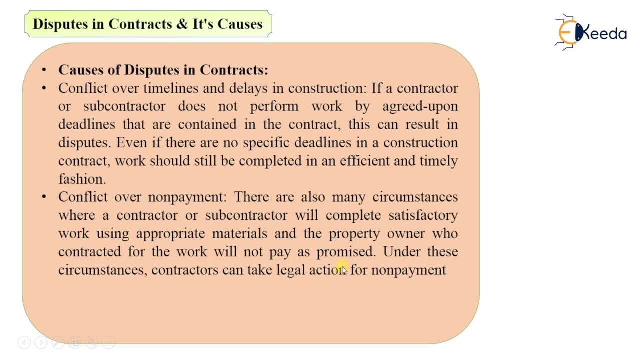 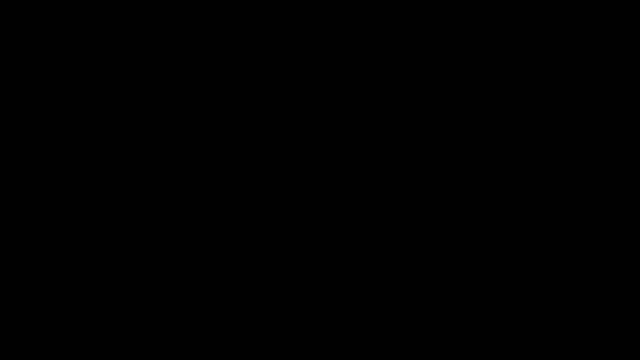 conflict between the owner and the contractor. So this was the video on disputes in contracts and causes of disputes in the contract. Thank you you.